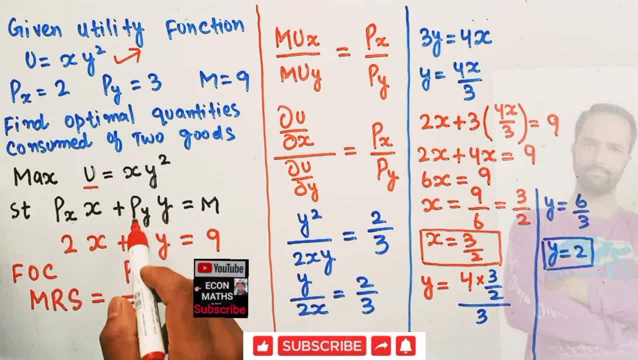 Okay. So we want to maximize utility of a consumer which is derived from the consumption of good x and y, subject to the budget constraint. What will be the budget constraint? Simple thing: price of good x times units of good x plus price of good y times units of good y should be equal to its income. That means income should be exhausted on the two goods. Okay, So price of x is being given as 2.. I have written here into x plus price of good y. 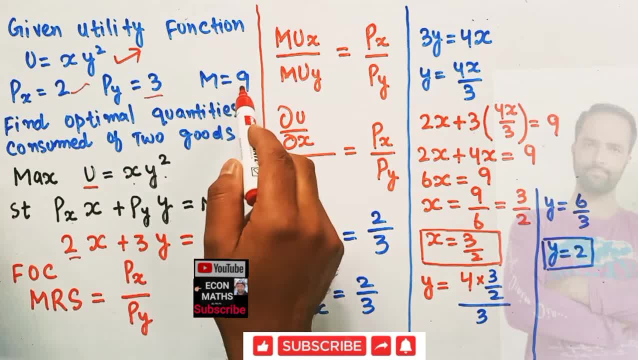 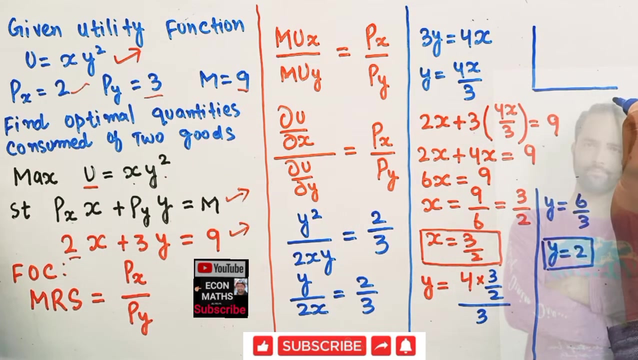 Good y is 3.. That's 3. y is equal to income of the consumer is 9.. I have written here 9.. Now first order. condition for optimization requires that modern rate of substitution between two goods, x and y, should be equal to their price ratio. Okay, Graphically it simply means, if I can draw the graph here. So the graph will look like this: Let us say we have units of good x on the horizontal axis, units of good y on vertical axis. Okay, 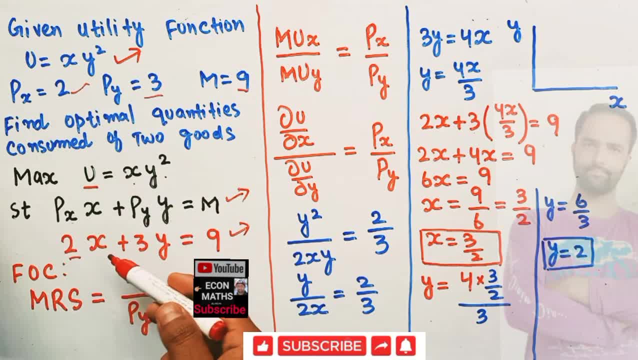 Okay, So we are being given the budget constraint. This, 2x plus 3y is equal to 9.. Let us say this is our budget constraint. First order condition requires that the modern rate of substitution between two goods should be equal to the ratio of the prices. So let us draw the indifference curve also here. Okay, So let us say this is our indifference curve. This, MRS, means simply the slope of indifference curve. Okay, Slope of indifference curve is our MRS. 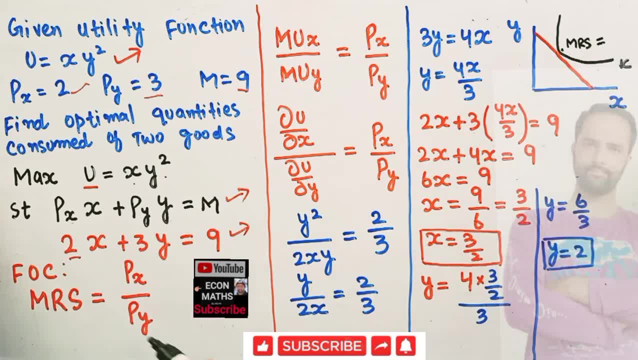 MRS, and it should be equal to the slope of the budget line, what we call the ratio of the price. Okay, It should be equal to the ratio of the price px upon py and graphically it means the point where our budget constraint or budget line is tangent to the indifference curve. corresponding to that point, we will have the optimal quantities of the two goods. Okay, So modern rate of substitution. 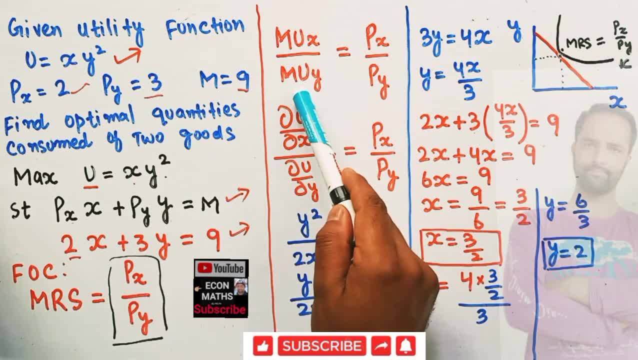 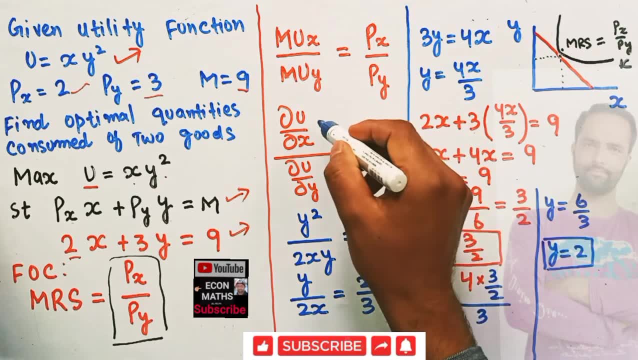 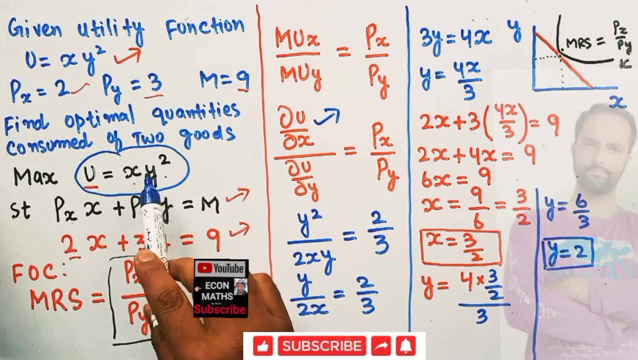 is equal to simply the marginal utility of good x upon marginal utility of good y should be equal to price of x upon price of y. Now, this marginal utility of good x means simply the partial derivative of our utility function with respect to x. If we take the partial derivative of this function with respect to x, derivative of x is 1.. So we are left with y square here. Okay, Similarly, du upon dy means the marginal utility of good y. 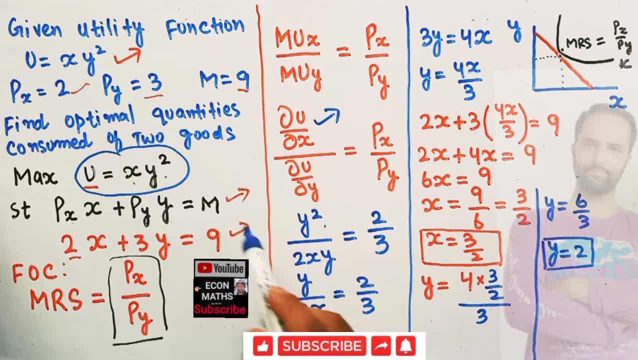 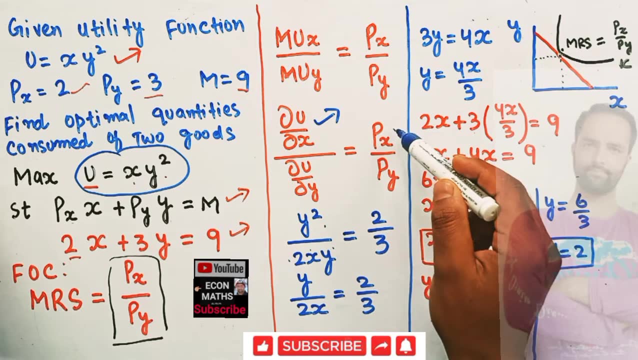 Okay. So this will come out to be, if we take the derivative of this function with respect to y. So this derivative of y square will be 2y, So we will get 2xy. It should be equal to the ratio of the prices. That means price of good x is 3.. Sorry, 2.. Price of good y is 3.. So this is equal to 2 upon 3.. Then we have, we can cancel 1y. here We are left with y upon 2x should be equal to 2 upon 3.. Solving for y: 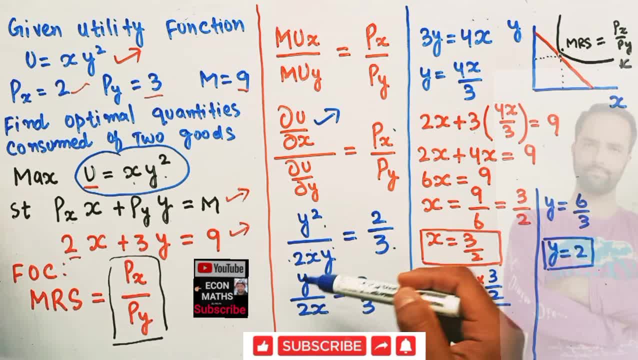 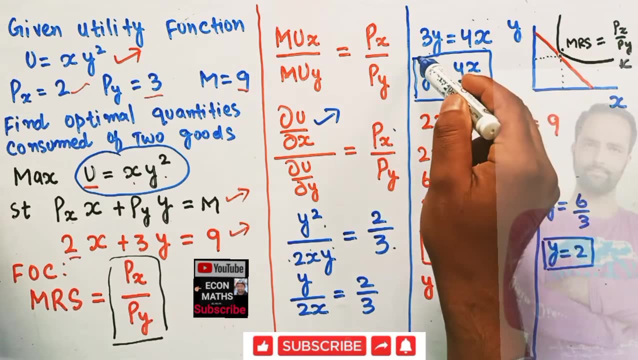 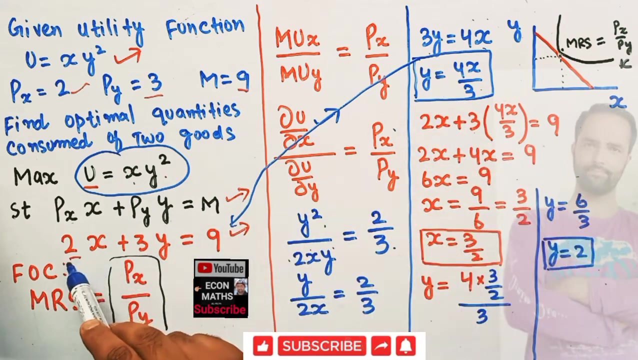 Okay, So we are multiplying this: 3y is equal to 4x. That means y is equal to 4x. Transposing this 3: here we get 4x upon 3.. Okay, Now what we need to do. we got the y is equal to this stuff. here We need to plug this value into the budget constraint. Okay, When we put the value of y into the budget constraint, we get 2x, as it is plus 3. in place of y, We write this value of y. 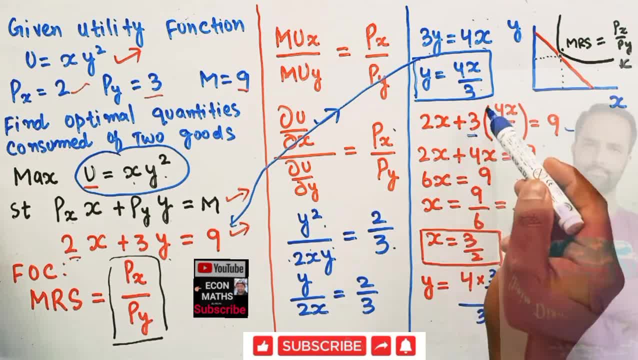 Y should be equal to 9.. So 2x plus this 3 and 3 will get cancelled. We are left with 4x here. So 2x plus 4x is 9.. That means 6x is equal to 9, which gives us x is equal to 9 upon 6, which is 3 upon 2.. That means optimal quantity of good x is equal to 3 upon 2.. 3 upon 2.. Okay, Now again we need to put the value of x is equal to 3 upon 2 either into our budget constraint or we can put 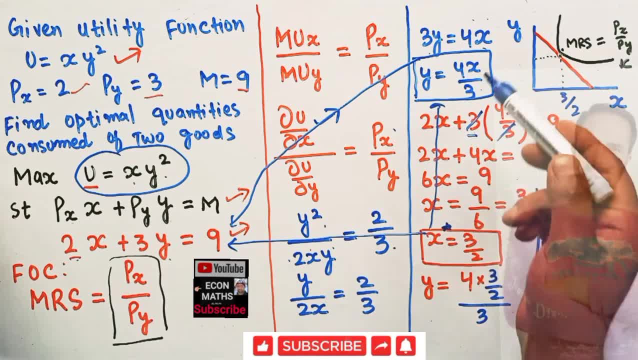 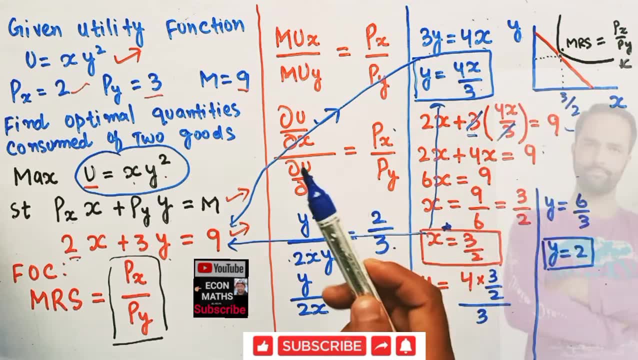 in this, where y is equal to 4x upon 3.. So I have just plugged. the optimal value of x is equal to 3 upon 2. in this equation You can put it back into the budget constraint, or in this equation. So it is your discreation here. Okay, So y will be.